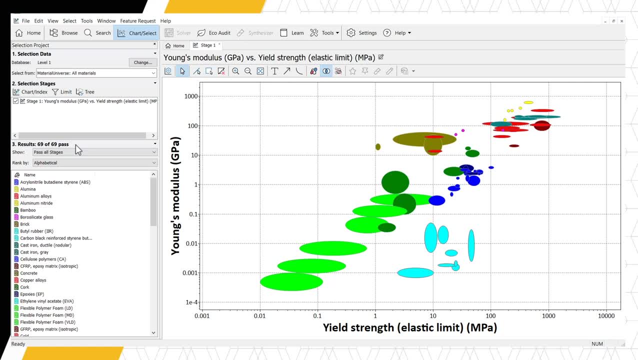 materials are suitable for our airplane wingspar. We want to consider all materials. for this selection problem, The results window simply shows all materials when a chart is made and no selection criteria has been applied. We want to investigate the stiffest and the strongest materials which are located in. 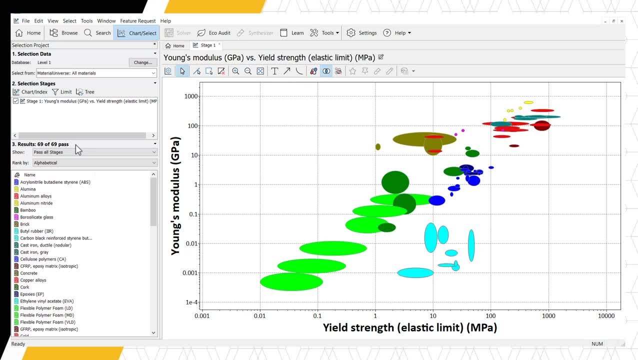 the upper right-hand corner of our chart To narrow down our material options. we can use the Box Selection tool from the chart toolbar and draw a box in our upper right-hand corner To narrow down our material options. we can use the Box Selection tool from the chart. 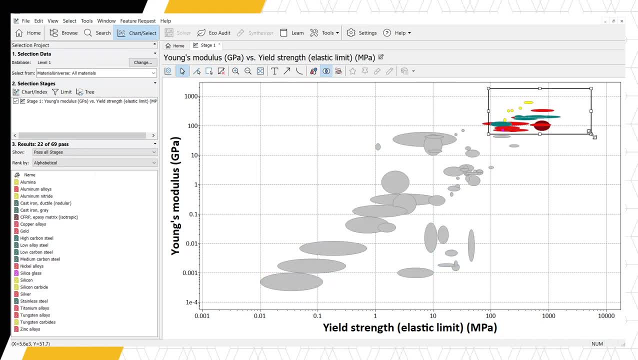 toolbar and draw a box in our upper right-hand corner. After drawing a box, we can select which material to select. After drawing this box, multiple things occur. First, the bubbles outside our selection box turn gray. This means these materials no longer meet our selection criteria. This is also 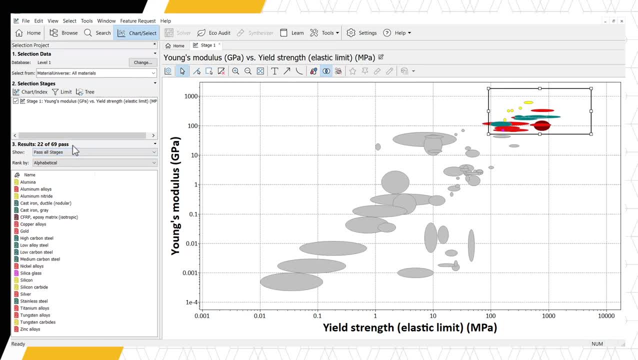 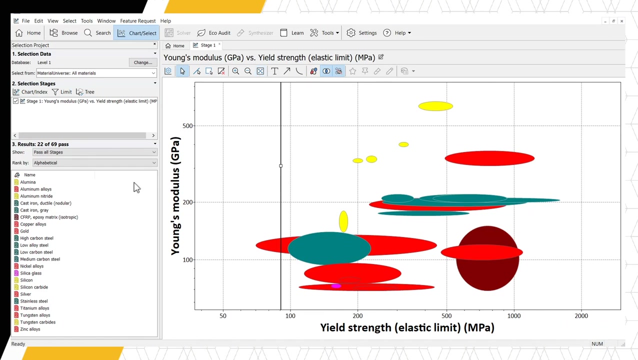 reflected in our results panel, where we now only have 22 materials that pass. For easier viewing, we can remove the gray bubbles using the Hide Failed Records button and auto-scale to zoom in on our current category. We can see from our results window that most of the materials that pass are metals or composites. 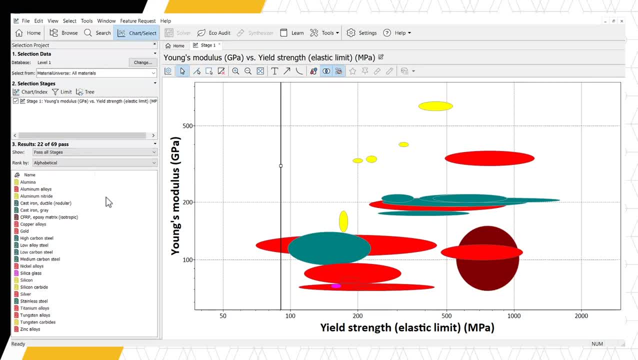 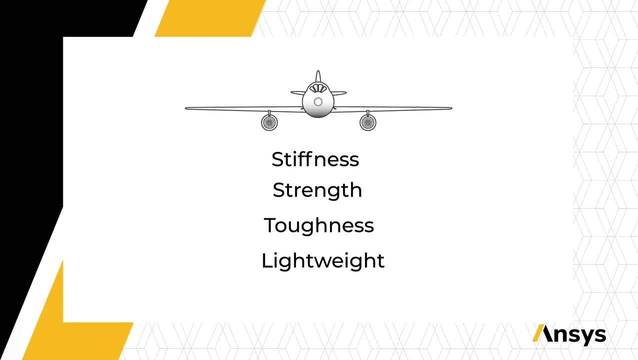 There are a few materials that do not make sense, For example, the yellow bubbles which indicate ceramics such as tungsten carbide, or the pink bubble indicating silica glass. To further narrow down our candidate materials, we need to look back at our selection criteria. 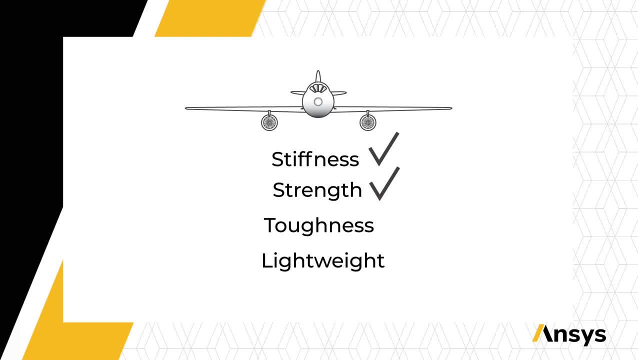 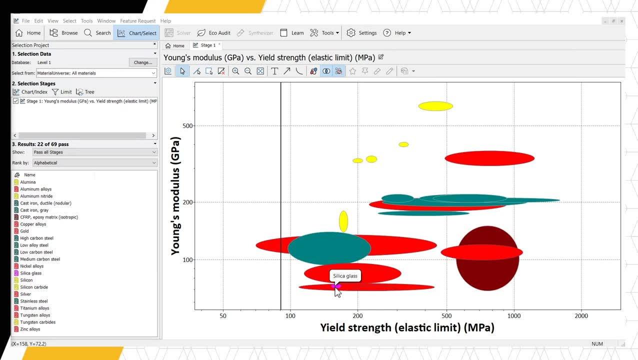 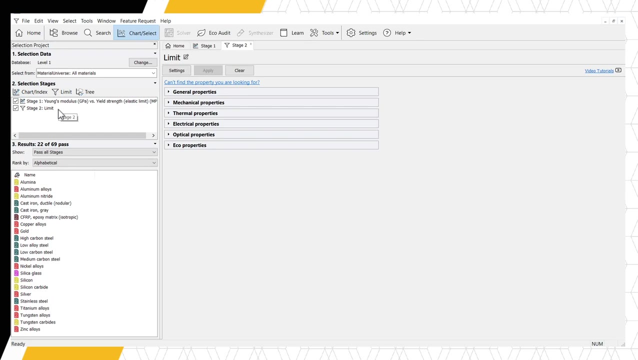 We have considered stiffness and strength so far. The next is toughness. We can apply this criteria with a Limit stage. Click Limit under Selection Stages to add a second stage to our selection project and go to Mechanical Properties. We can see from the small graph icon next to Fracture Toughness that metals and composites have the highest. 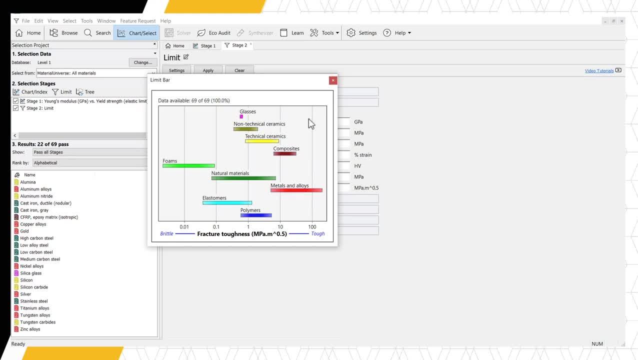 fracture toughness of our available material factors. We can see from the small graph icon next to Fracture Toughness that metals and composites have the highest fracture toughness of our available material factors. This means that the partially-dest converged metals are now available in the larger sample of our Undi breve. 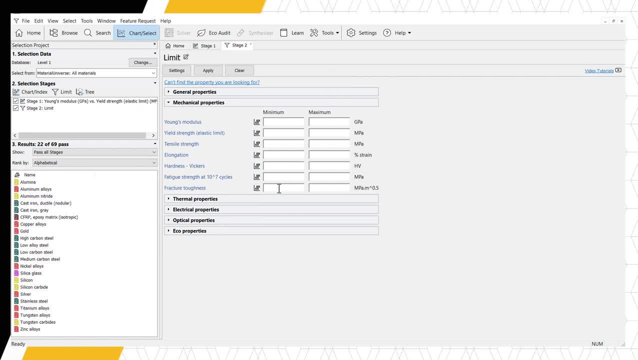 aqueles so we can choose. choosing from the multiplealloth families, Let's select a minimum of 10MPa flag respectively for our Fracture Toughness and click Apply. We can already see that in our result window we went from 22 to 16 materials, passing all stages. 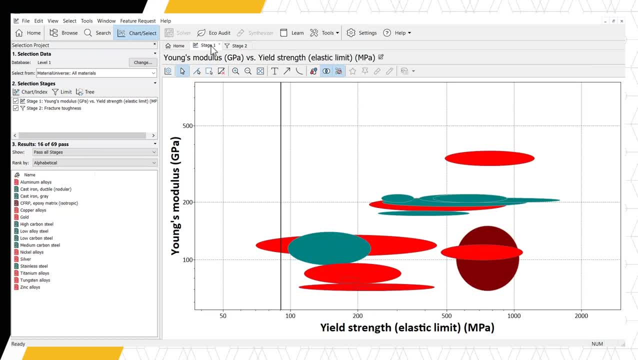 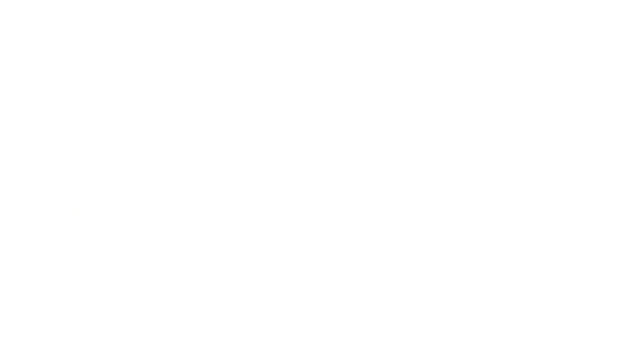 Going back to our chart, stage 1, using the tabs at the top of the screen, we can see that the Ceramics and Glasses have been removed from our chart. We have now considered three of our criteria: stiffness, strength and toughness. The last consideration is materials that are lightweight or have a low density. 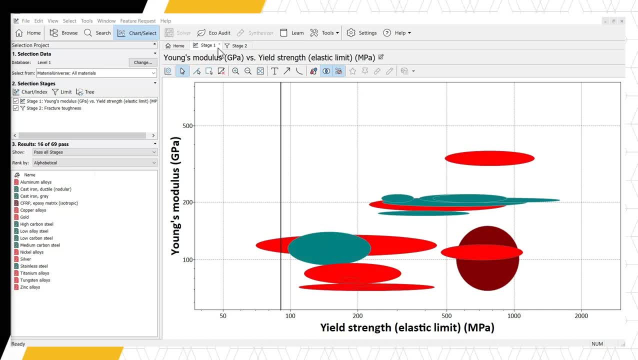 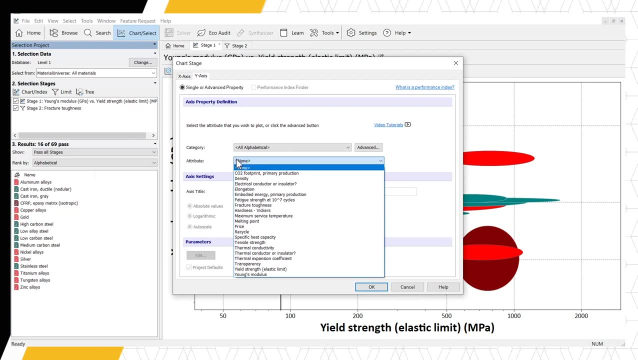 To consider density. let's create another chart within the same project to look at our candidate materials against different criteria. For the y-axis, select density. If we were going to manufacture this plane, another consideration would be price. So, using the tabs at the top of the chart window, again choose the x-axis and select. 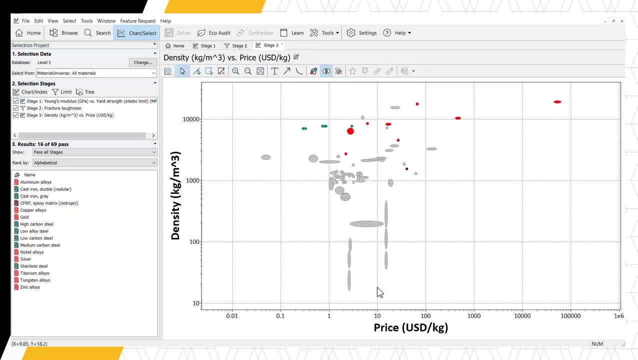 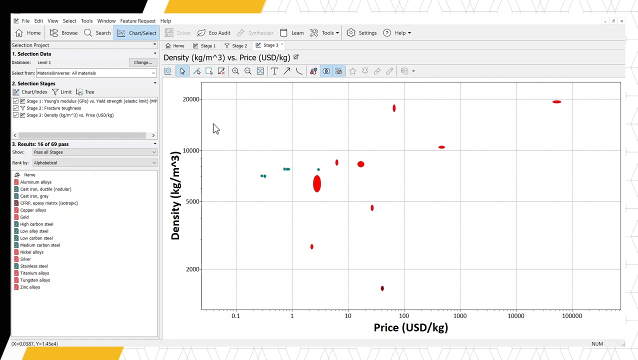 price. Click OK to generate the chart Automatically. all materials, including the ones that do not pass our previous selection stages, are shown. We can once again hide these failed records and auto scale. At this stage in our selection, we are trying to optimize our results and look at this trade. 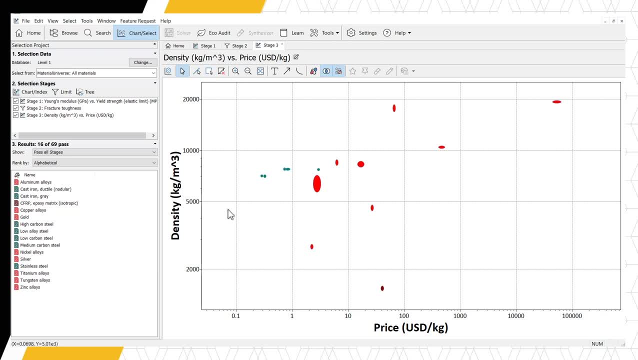 off between density and cost. If we are mainly concerned with low density, carbon fiber composites are our best material candidate. If we are mainly concerned with low cost, cast iron would be our best material candidate. If we want to balance, we can select the material in between the two. 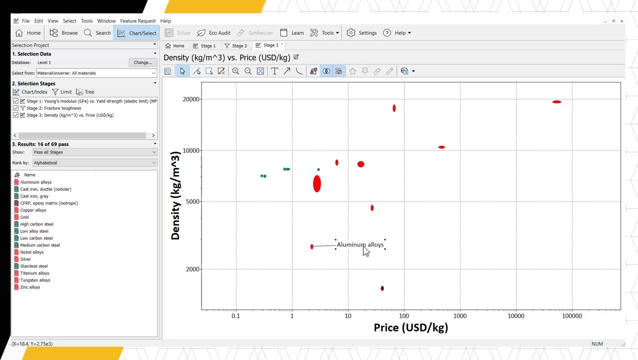 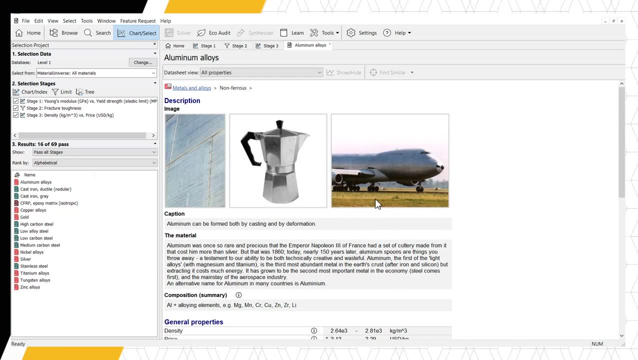 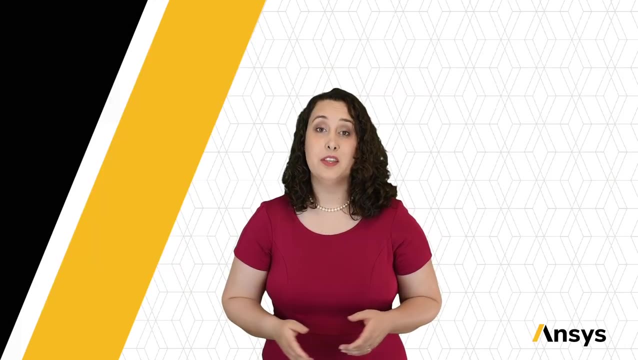 Aluminum alloys. Opening this data sheet by double-clicking the record shows us some example uses, at the top one of which is an airplane. This gives us additional confirmation that we have selected a sensible material. In this how-to tutorial, we've demonstrated how the material selection. 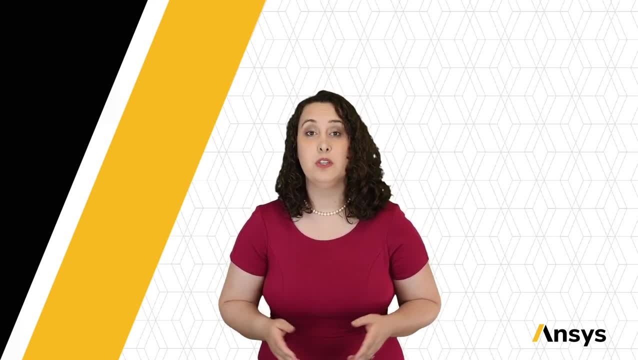 tools within our Granta EduPak software can be used for material selection based on product criteria. For more information on Granta EduPak, check the link in the description. Be sure to check out our channel for more ANSYS learning videos, and thank you for watching.